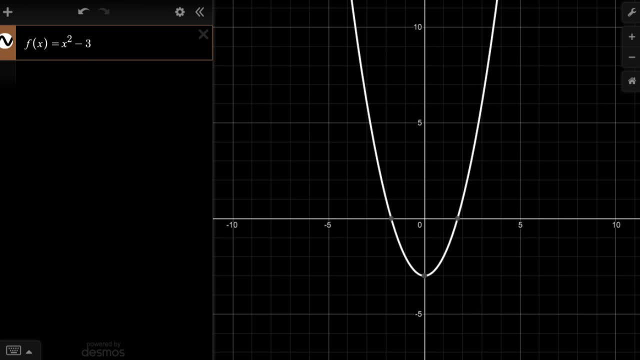 And we can set up a slider here to make that a little bit clearer. So if I just replace this with, if I just replace this with the variable k, then let me delete this little thing here, that little subscript thing that happened. 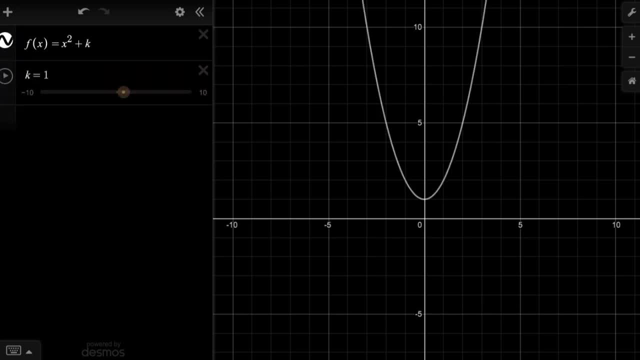 Then we can add a slider k here, And this is just allowing us to set what k is equal to. So here k is equal to one. so this is x squared plus one. And notice we have shifted up. And if we increase the value of k, 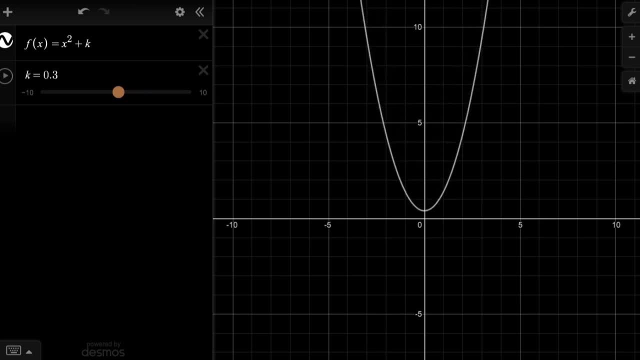 notice how it shifts the graph up And as we decrease the value of k. if k is zero, we're back where our vertex is right at the origin, And then, as we decrease the value of k, it shifts our graph down, And that's pretty intuitive. 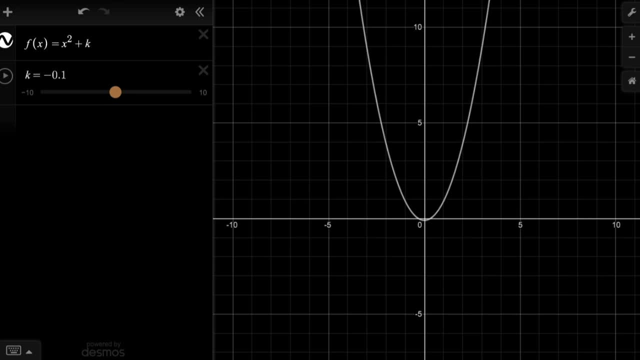 because we're adding or subtracting that amount to x squared, so it changes, we could say, the y value. It shifts it up or down, But how do we shift to the left or to the right? So what's interesting here is: 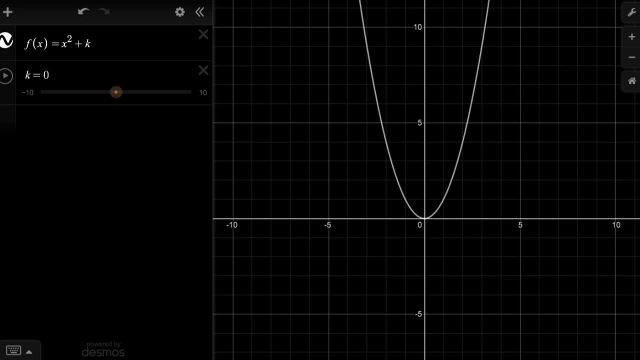 to shift to the left or to the right. we can replace our x with an x minus something. So let's see how that might work. So I'm going to replace our x with an x minus. let's replace it with an x minus one. 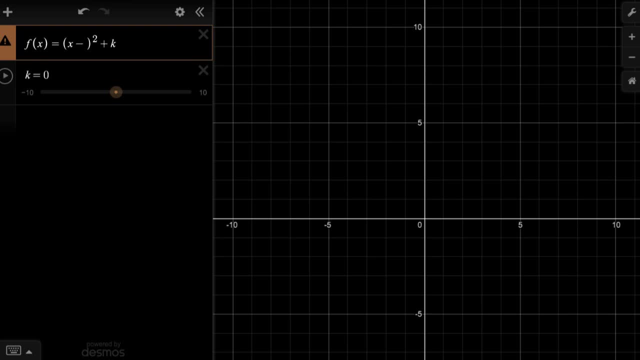 What do you think's going to happen? Do you think that's going to shift it? one to the right or one to the left? So let's just put the one in. Well, that's interesting. Before, our vertex was at zero: zero. 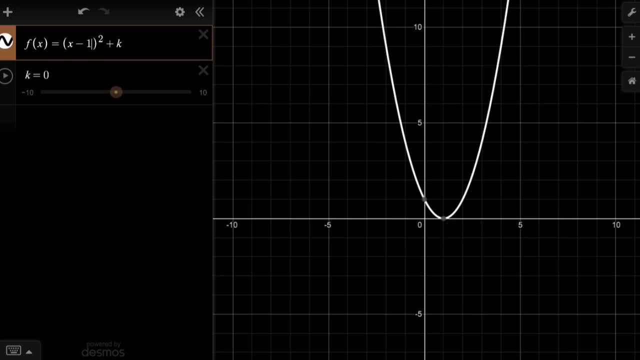 Now our vertex is at one zero. So by replacing our x with an x minus one minus one, we actually shifted one to the right. Now, why does that make sense? Well, one way to think about it before we put this x. 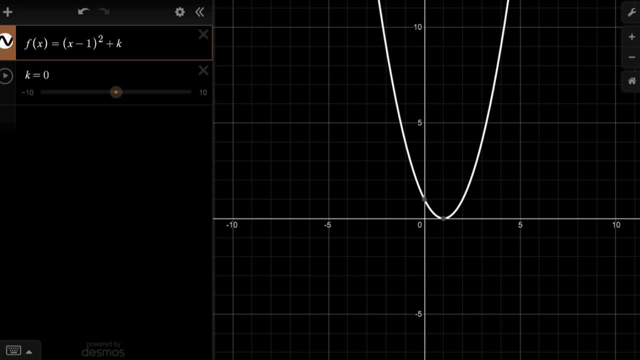 before we replaced our x with an x minus one, the vertex was when we were squaring zero. Now, in order to square zero, squaring zero happens when x is equal to one. When x is equal to one, you do one minus one. 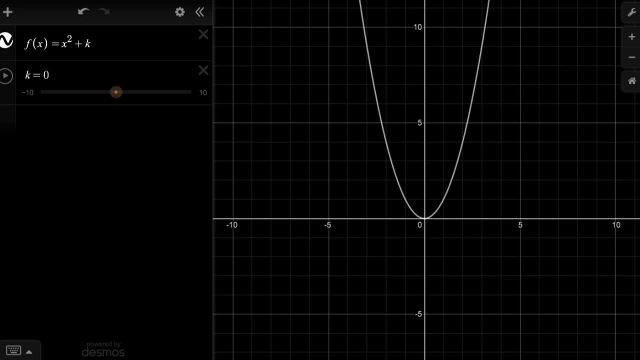 to shift to the left or to the right. we can replace our x with an x minus something. So let's see how that might work. So I'm going to replace our x with an x minus. let's replace it with an x minus one. 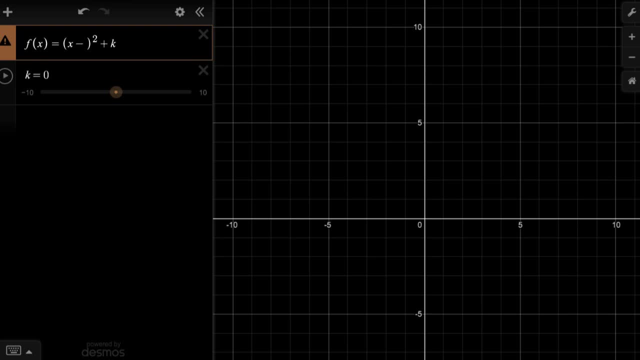 What do you think's going to happen? Do you think that's going to shift it? one to the right or one to the left? So let's just put the one in. Well, that's interesting. Before, our vertex was at zero: zero. 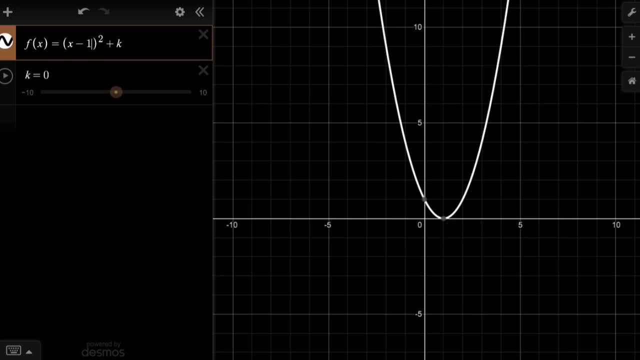 Now our vertex is at one zero. So by replacing our x with an x minus one minus one, we actually shifted one to the right. Now, why does that make sense? Well, one way to think about it before we put this x. 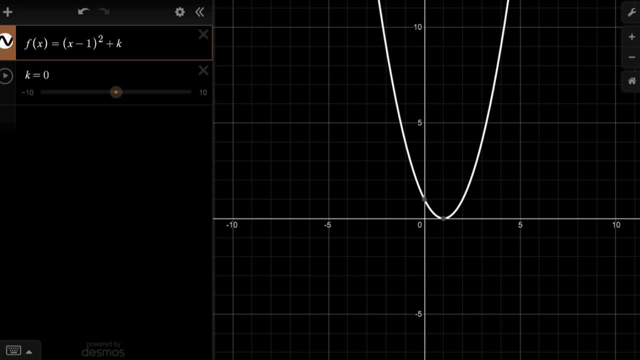 before we replaced our x with an x minus one, the vertex was when we were squaring zero. Now, in order to square zero, squaring zero happens when x is equal to one. When x is equal to one, you do one minus one. 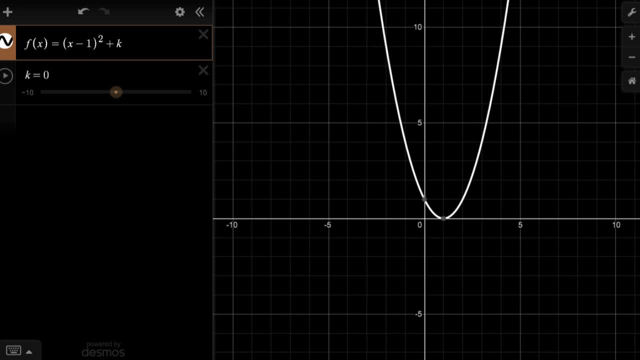 you get zero, and then that's when you are squaring zero. It makes sense that you have a similar behavior of the graph at the vertex now when x equals one, as before you had when x equals zero, And to see how this can be generalized. 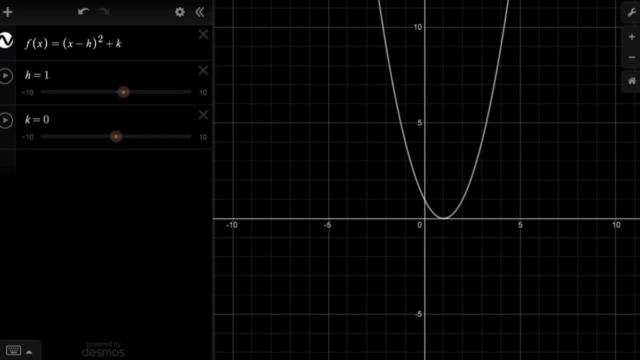 let's put another variable here and let's add a slider for h, and then we can see that when h is zero and k is zero, our function is really then just x squared, and then, if h increases, we're replacing our x with x minus a larger value. 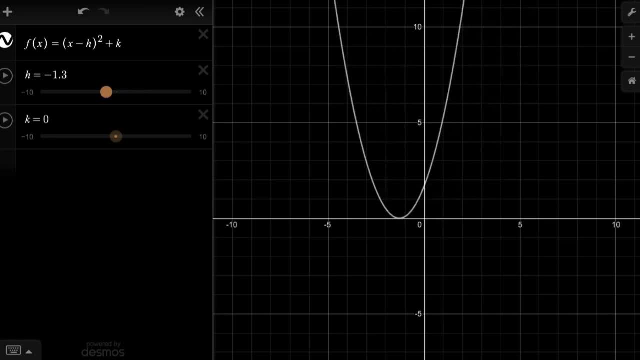 That's shifting to the right. That's shifting to the right And then, as h decreases, as it becomes negative, that shifts to the left. Now, right here, h is equal to negative five. You typically won't see x minus negative five. 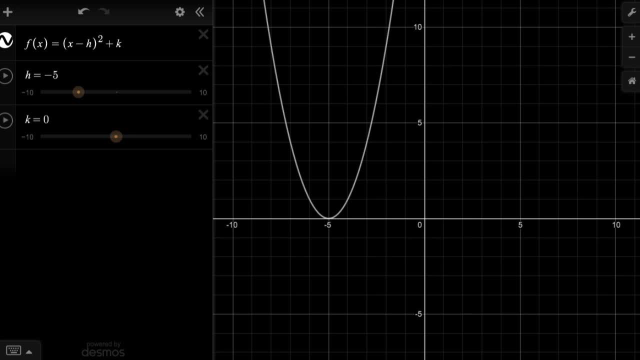 You would see that written as x plus five. So if you replace your x's with an x plus five, that actually shifts everything five units to the left, And of course we can shift both of them together like this. So here we're shifting it up. 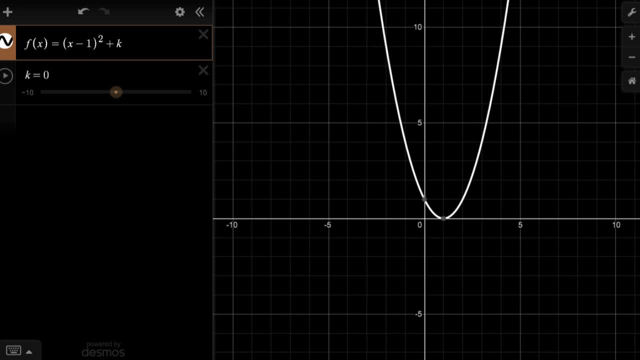 you get zero, and then that's when you are squaring zero. It makes sense that you have a similar behavior of the graph at the vertex now when x equals one, as before you had when x equals zero, And to see how this can be generalized. 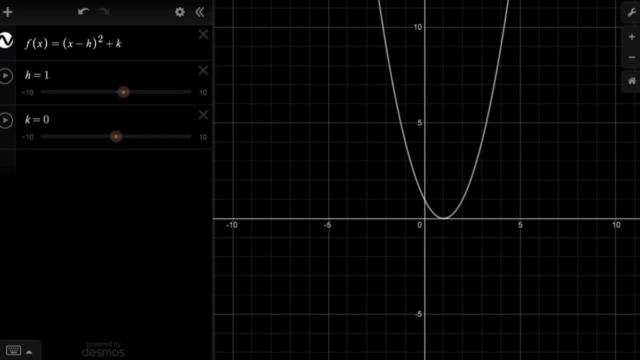 let's put another variable here and let's add a slider for h, and then we can see that when h is zero and k is zero, our function is really then just x squared, and then, if h increases, we're replacing our x with x minus a larger value. 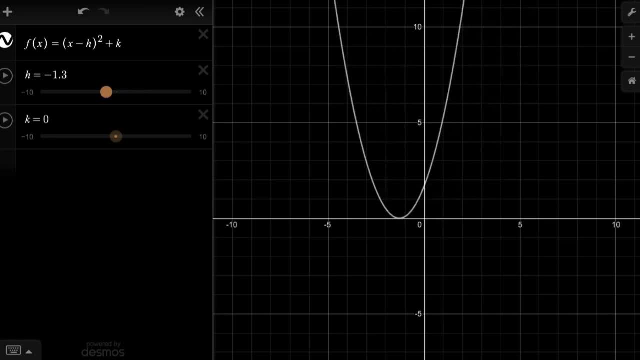 That's shifting to the right. That's shifting to the right And then, as h decreases, as it becomes negative, that shifts to the left. Now, right here, h is equal to negative five. You typically won't see x minus negative five. 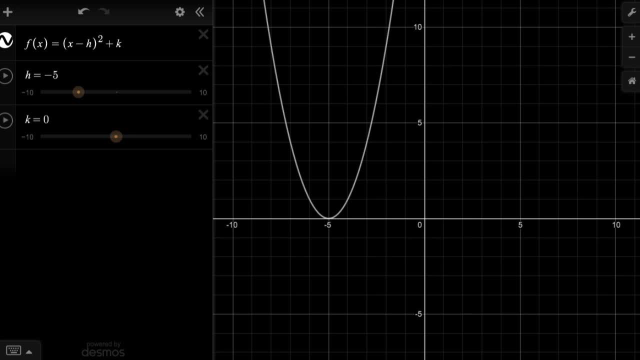 You would see that written as x plus five. So if you replace your x's with an x plus five, that actually shifts everything five units to the left, And of course we can shift both of them together like this. So here we're shifting it up. 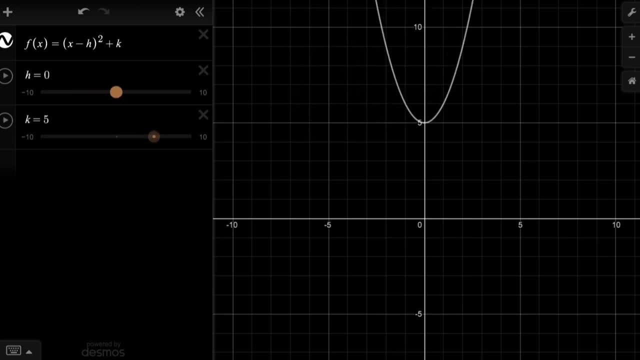 and then we are. we could get back to our neutral horizontal shift and then we can shift it to the right, like that, And everything we did just now is with the x squared function as our core function, but you could do it with all sorts of functions. 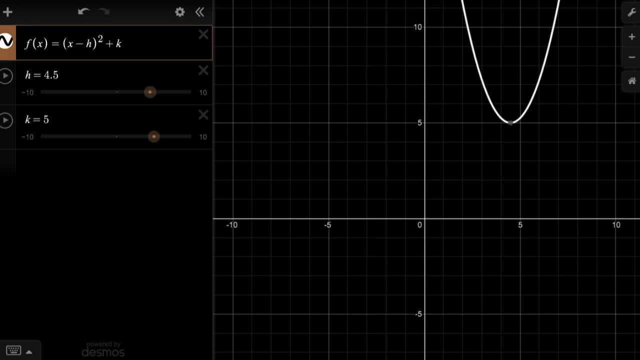 You could do it with an absolute value function. Let's do absolute value. That's always a fun one. So instead of squaring all this business, let's have an absolute value here. So I'm gonna put an absolute whoops, absolute value. 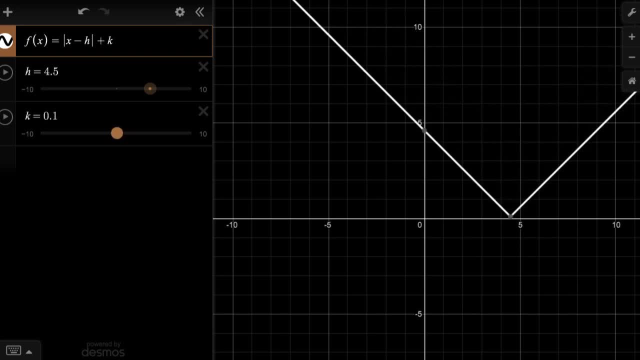 And there you have it. You can start at. let me make both of these variables equal to zero. So that would just be. the graph of f of x is equal to the absolute value of x, But let's say you wanted to shift it. 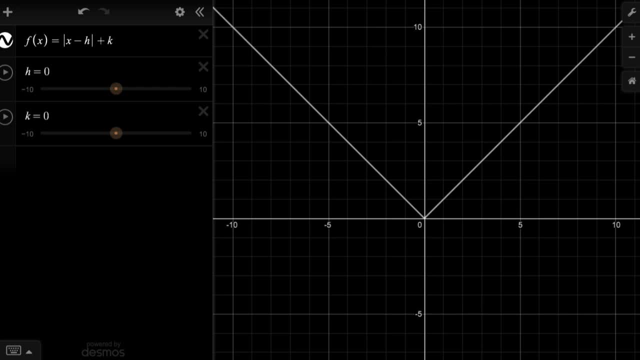 so that this point right over here, that's at the origin, is at the point negative five, negative five, which is right over there. So what you would do is you would replace your x with x plus five, or you would make this h variable.